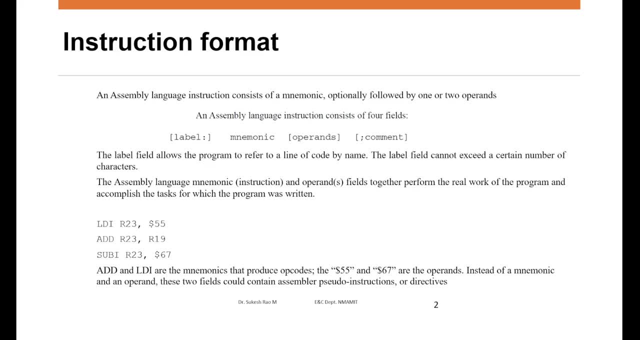 aspect of an assembly language, so how an assembly language looks like. assembly language instruction will consist of some mnemonics, so they are the english type of statements, and in generally in assembly language will contains this. the field number one: this is label and you have mnemonic and operands and comments. there are four different fields: what the label is. label is usually. 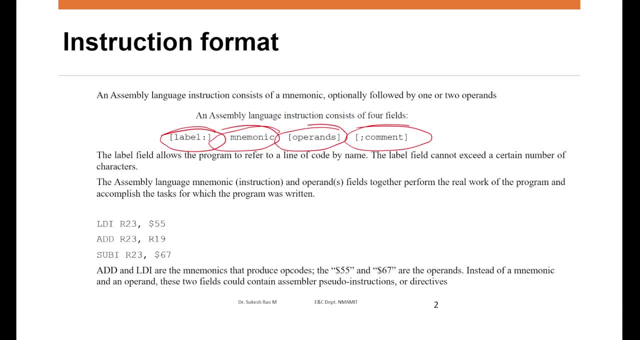 you know it is a kind of you know marking that we use in case of loop like, for example, i need to make an instruction to come to this location, then i use it as a label. usually it is treated as an you know address. in the instructions mnemonics are the statements like an, which indicates that an operation, for example, 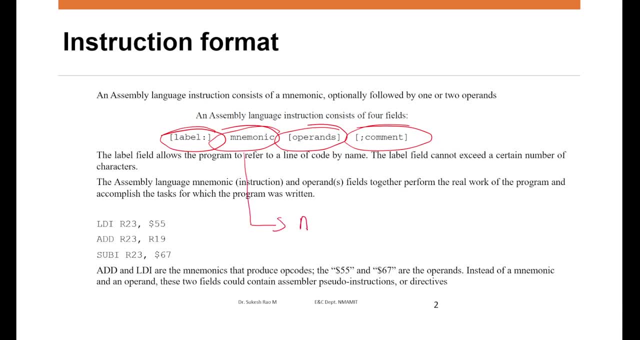 i can have a mnemonic as, let's say, add, so add means i'm adding. then you have, say, sub, you are subtracting. then you have rotate, you may be rotating. okay, these are some of the instructions which indicates you know what is that instruction supposed to do. you get to know what that instruction within mnemonic. 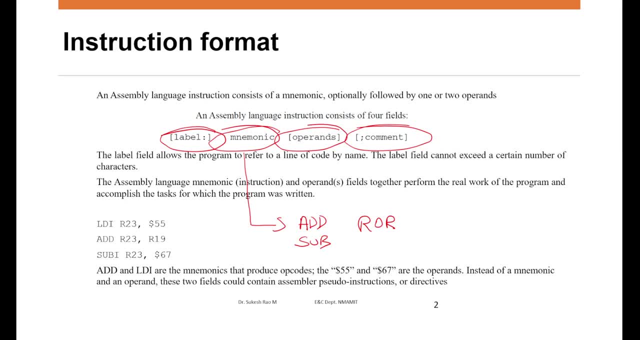 obviously, along with the mnemonic, i should feed certain parameters with to the operation, like add what to add, to subtract what to subtract, or if you want to move something from way to move. so that is what is called as an operand. so we should fill that operands. so operand fields are like this: these are all operands. 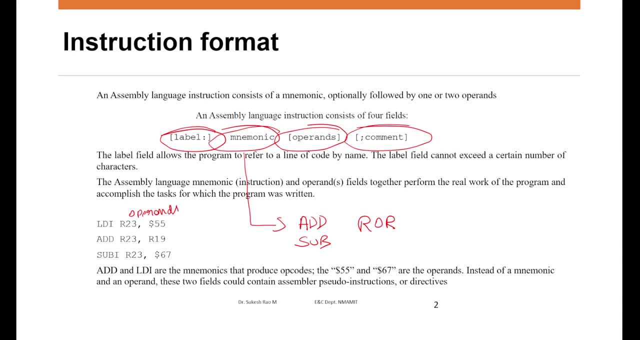 these are all operands, like r23, hash 55. no, these are all the operands. if you look at this, here it is ldi: r23, dollar 55. now, what it does, is it? uh, now, here, this is the mnemonic, this is the operands. now, this operands will tell you're loading some register r23 with the value 55, that's what. 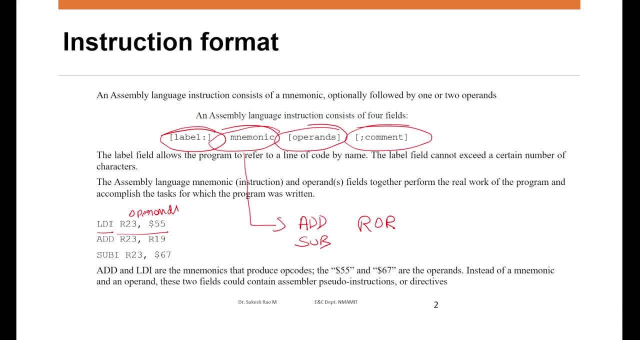 let's say there are at 10 parameters. then i supposed to load that 10 parameters to the 10 value, 10 to some register. so i use ldi instruction. so these are all operands here. similarly, add: you can straight away think about what is to be added. so it's given 23 and r19. so let's see the working of this in detail. but 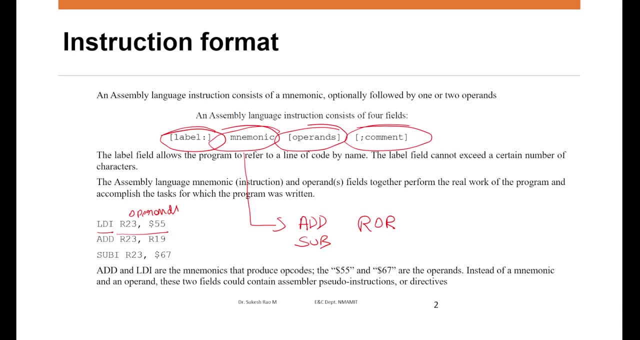 the typical, uh, you know, usage of an assembly instruction will have these operands. comments are usually given, you know, optionally to indicate: okay, you know what is the operation of the mnemonic mnemonic, i am sorry. okay, what is the operation of the mnemonic Sketcher, etc. you have to start. 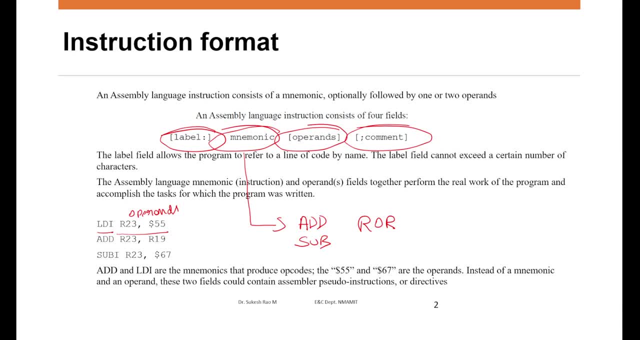 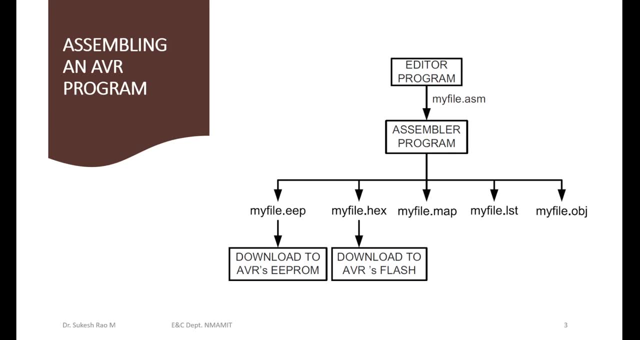 counting yourself out here. okay, if you have this mnemonic, take this box, let's say PC in g 국민 shook, Removing and completing the mnemonic. that's like when you do something, for example the mnemonic one, because you signal other mnemonic. the problem is that 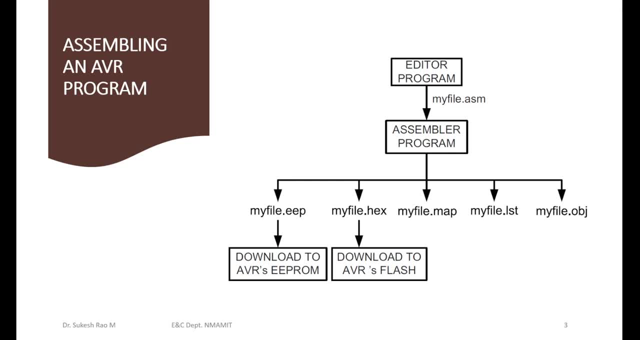 you will do everything differently so you can, Sundays, will come up with different types, Curry rows or times and other hygiene options, so it actually can solve that. we will go ahead and we will solve sci-fi problems of libel maneuver. those folks can come up with some sort of problems. 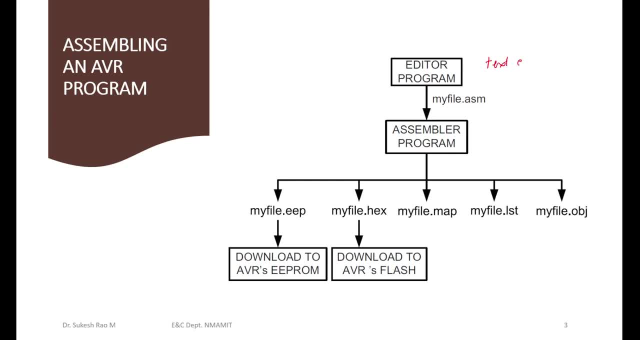 of inferiorityMcL mest will be not safe because that will. beagna system helps us to process that. I may use some text editor here. So if you open any text editor and you type the code, So you should follow certain. you know the format of writing the assembly instructions and some. 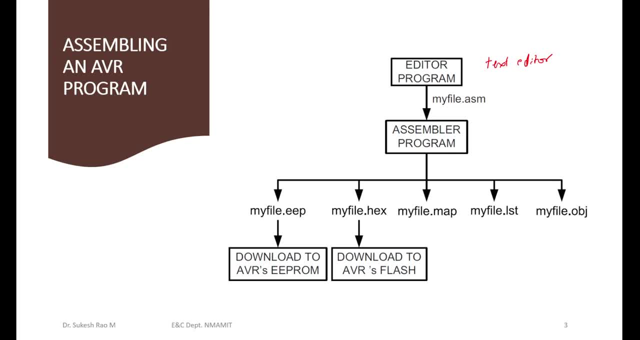 header files may be have to include it, depending on which assembler you are using. So usually any word processor or a text editor I can use to edit that program and usually extension of that assembly file is dot ASM. So if I, if you find some file with dot ASM, it indicates that 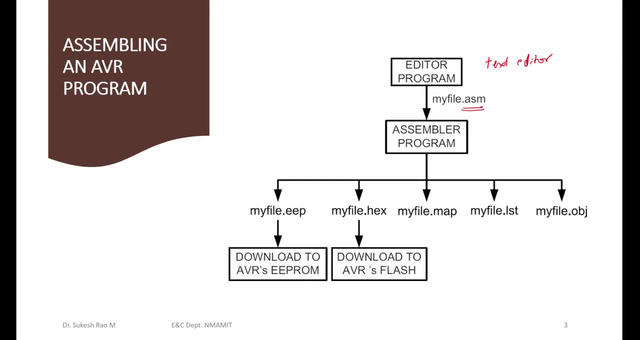 it is an assembly file, So from that assembly file I should compile it to another file, because this ASM file your processor even does not understand if I write add R23, comma R16. it cannot understand what this instruction is, So cannot understand by the controller, because it is an English type of statement, what it can. 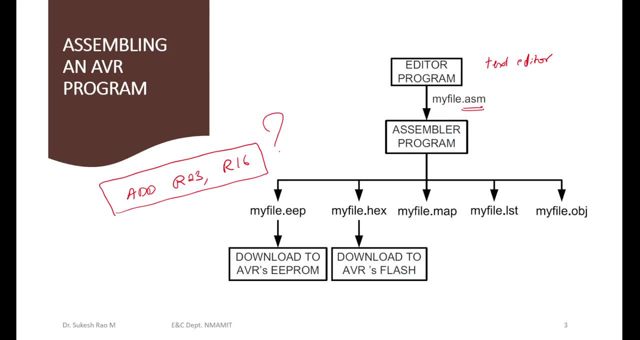 understand. as I already mentioned, it understand only the binary numbers. So how do you compile from this to some binary? that is what this assembler does, So it converts this to some number. let us say this converted to C256 and just taking one random example. So this is actually. 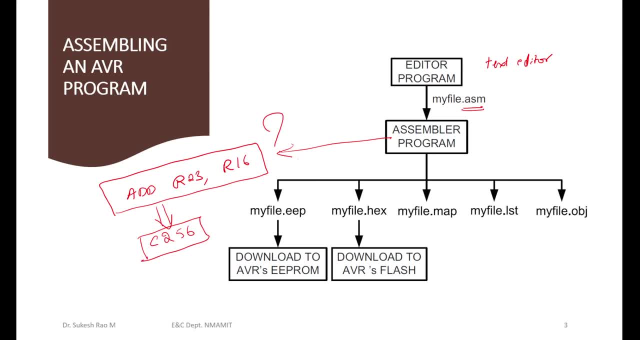 this instruction is coded as C256.. So C256, you write in bit. So that is what the content of this hex file. So this hex file will contain the C256 which is corresponding to this. that is the hex file. So, apart from that, there, 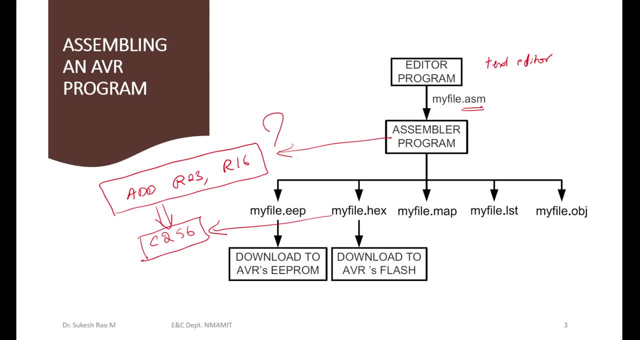 are. some other files are generated, which we will see what is the content and why it is. And there are again one more file. you can see EPP. this is EEP, which is actually used to flash the code into some EEPROM memory, because your controller will also have some EEPROM memory. 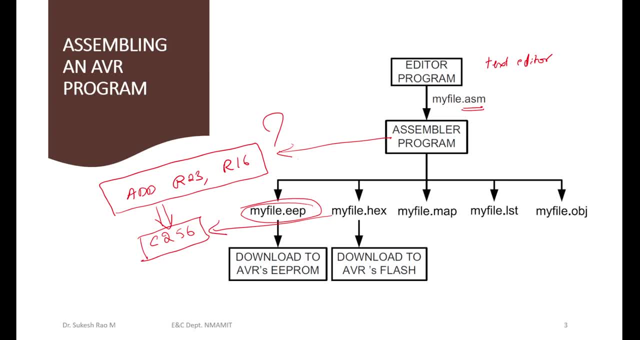 So you have an EEPROM where you want to store certain configurations or any other data which you wanted to be there permanently. then we go for EEPROM memory. there is a way of compiling and you get it as EEP. The main intention of come assembling is to get the hex file. 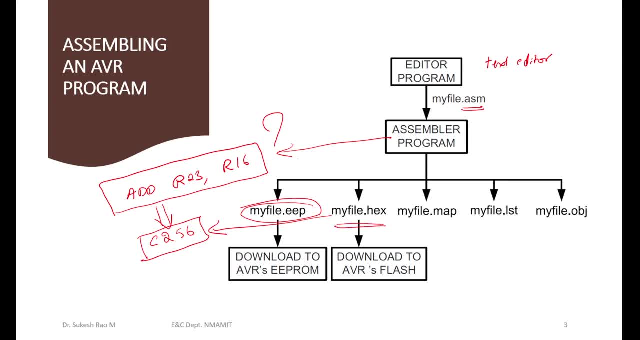 this is something, target file. what is a binary file? or a hex file, some case? So hex file is required, which is usually in numbers which can be only understood by the controller. we cannot even Cross compile it. it is very difficult to cross compile a hex file. back to the assembly: nobody. 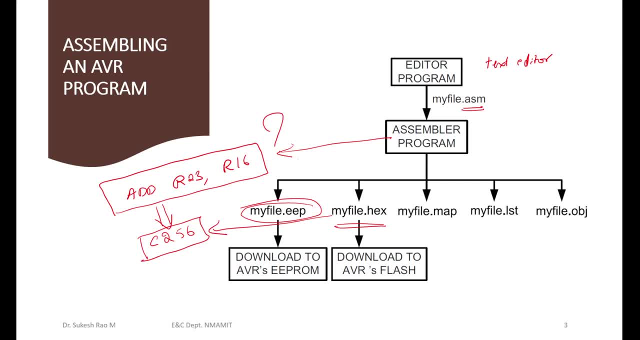 does it to, and it is. it is actually coded in this way. Apart from that are a map file, list file, object file and usual procedure means C. also, we do the same way of compilation from a high level language to a machine language. If you look at the content of the list file, it 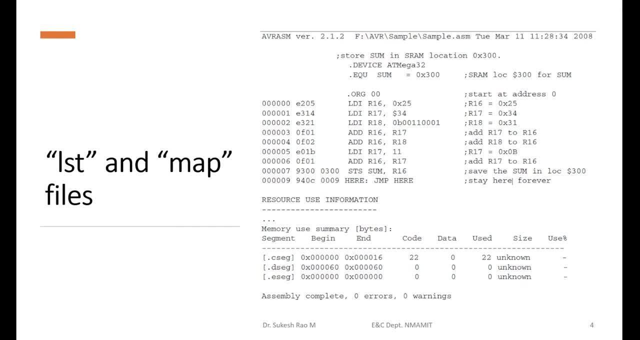 has a lot of informations, like each instructions which memory is saved and you can have some look at this instructions here. like you have LDI R16, 0X-25.. So this is loading a number: R16 to 25, so that's how it is indicated. so if you look at this instruction, you can see. 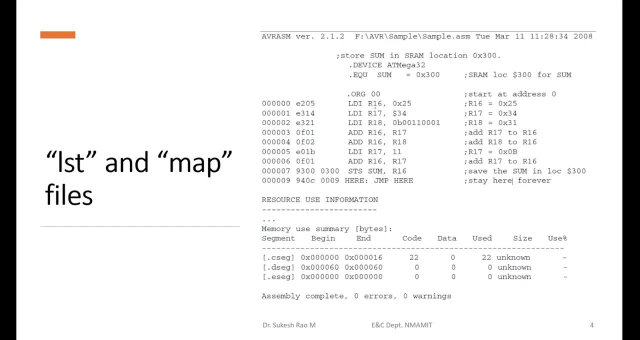 this is the mnemonic. ldi is a mnemonic. r16 is the operands. 0x25 is another operand, but you look at this, it is written as some code here. this is what x code, what i get in the hex file and this is the program memory, correct? this is the program memory location where this number. 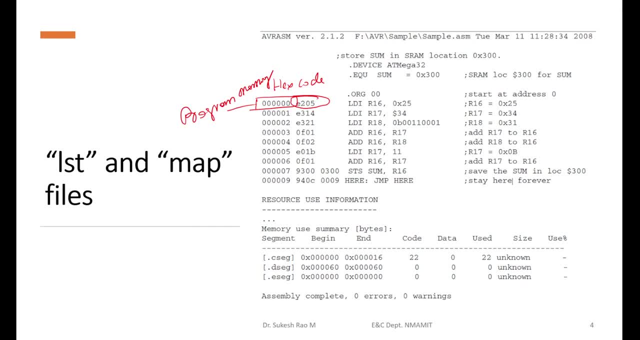 is saved. so in each locations- and it's a word data, okay, in one location a 16-bit value is saved. that's why the next location will have another 16-bit number. next location, another 16-bit number. so in each locations you are going to have some opcodes for the hex codes. that is what. so your 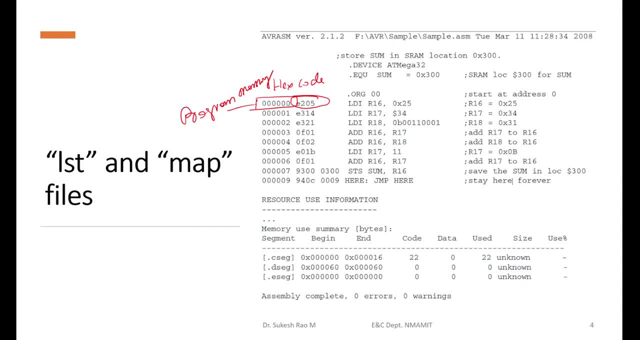 your list file will give you the complete detail of how it is organized and here you can say: this is a label, what we say, this is a label, so this is a label, so this is a label, so this is a label. label indicates I am jumping over here and here is actually the address. what is. 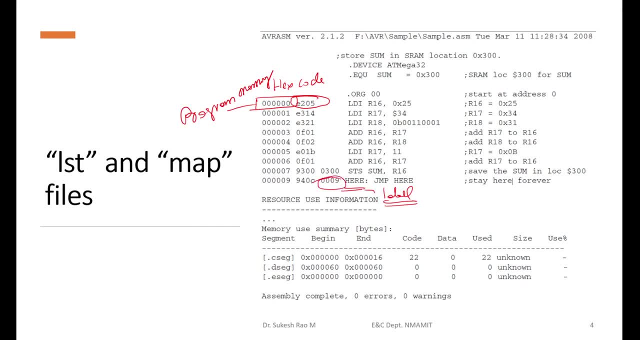 that address. this is address, here is address and usually in in. you know, when we compile it to get hex file, usually these labels are replaced with the address. so, and apart from that, you can also seek some comments. you can see these are all the commands that we write. so commands are also important. we will come. 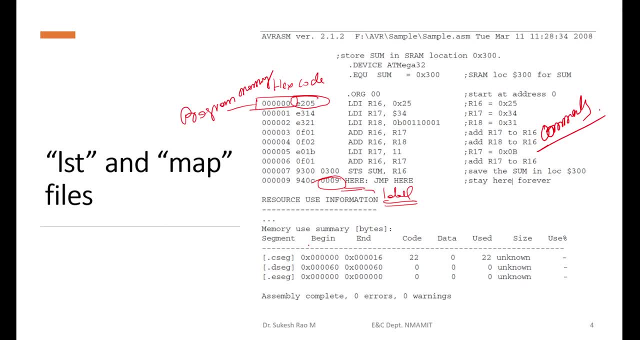 to know, okay, what does instruction does. and also you can find some memory usage. okay, this will indicate some memory related. and finally you get something information about the assembly, a note like: if there is zero error, zero warning, okay, these information. so sometimes we may have to see some information in the 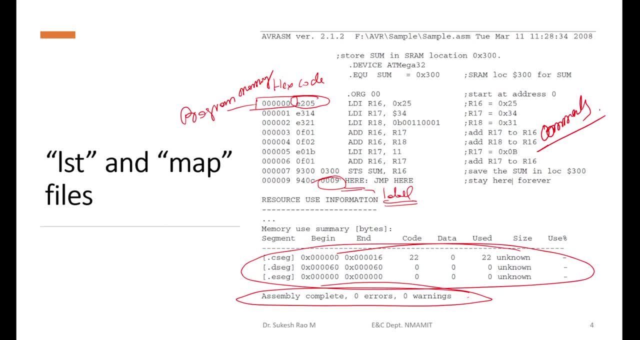 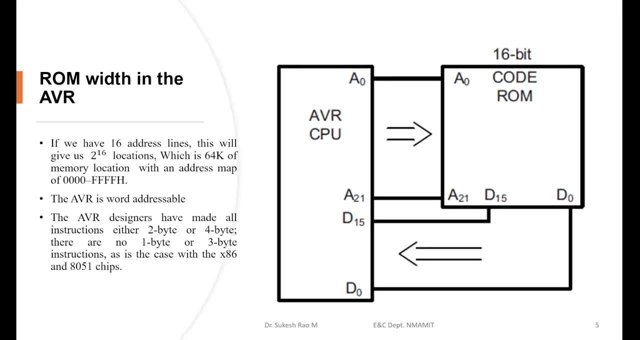 list file to see what exactly is happening in the memory or maybe the warnings information, okay, these things. so now, so we know now how we can use this information in the assembly. so now, so we know now how we we can use this information in the assembly. so now, so we know now how we. 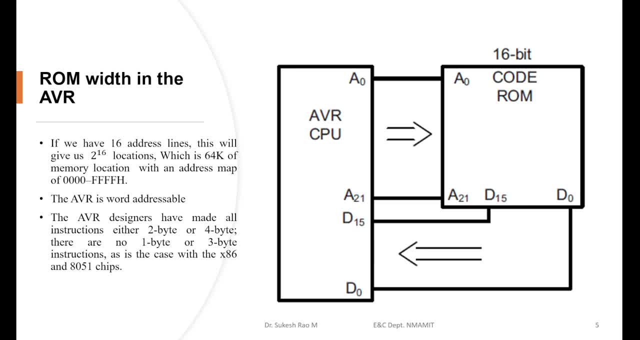 the process is, you know, involved in assembling program from the assembly to hex and what are the files are generated using the assembly? now let's look into the some memory aspect of a processor here. so this is the avr central processing unit and I can see some 22 address lines are here and 16 data lines. 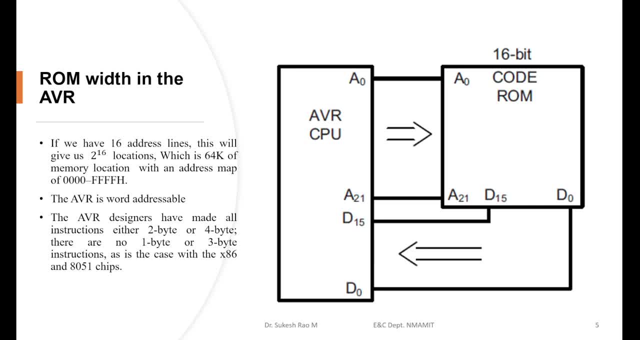 are there now. a typical controller may have some restricted amount of memory so, like in this example, it is 64k. So 64k actually needs only 16 address lines. So if I have some number till a 15, then I will be having 16 lines. ok, So 16 lines means I will be having 2 to the 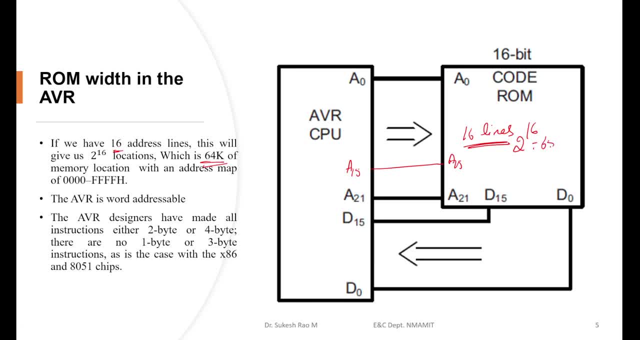 power of 16 locations, which is 65,064. yeah, 64,536, 64,535. ok, This is a number that I get, 2 to the power of 16.. So, which is called as. I guess this is 65,535 and this is called as. 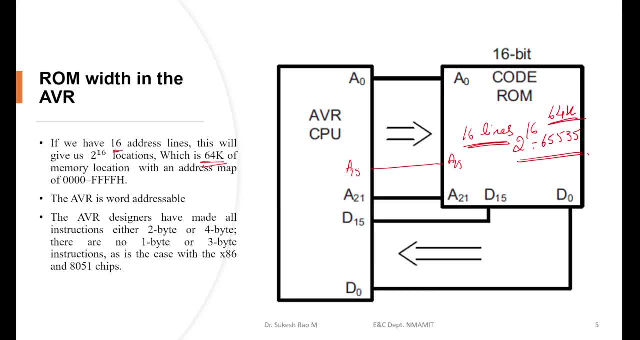 65,535.. So this is called as 65,535 and this is called as 65,535.. So this is called as 64k. ok, standard memory it is. So there are these many locations. 65,535 locations are there. 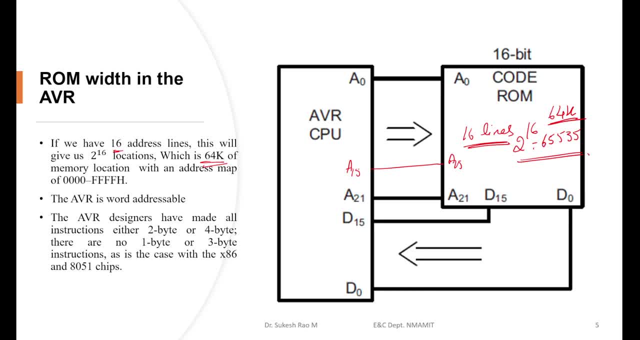 Now in each location, how many bits of data is saved. Just concentrate, just focus here in each location, how many bits of data It is here. in this case, it is 16 bit data. It is a 16 bit of data that is saved Now. this is actually the code memory. 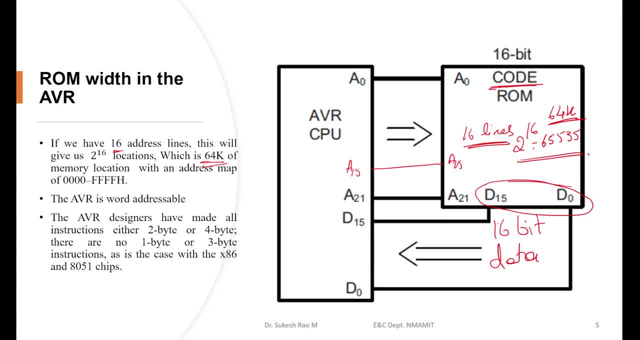 Ok. So, and the beauty is here, each code is 2 byte most of the time. Sometime it may be 3 byte, 4 byte. sorry, but it cannot be an attributed value like 3 byte, 1 byte. No, that is not. that is not. 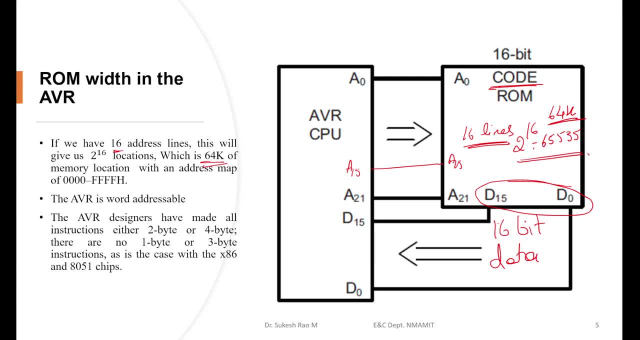 there. So in AVR, any instruction you take, either it takes 2 byte or it takes 4 byte. That is how this memory is actually. you know the number of cycles. Ok, That is why it is required, for the execution is mapped. So if you are using the, since the 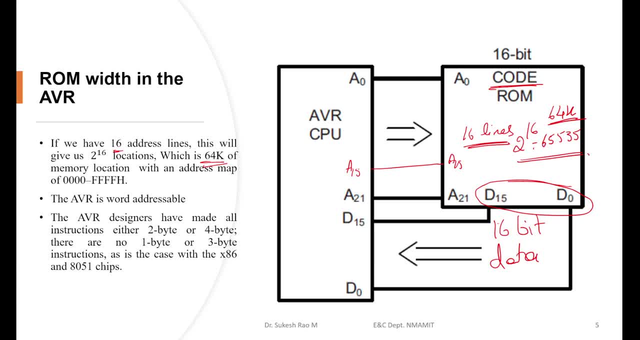 memory is actually restricted in the even numbers like 2 byte, 4 byte, 6 byte, so on. So it is not possible to it is not feasible to have this 1 byte, 3 byte location, So usually the instructions also coded is also 2 byte or sometime it is another 2 byte. 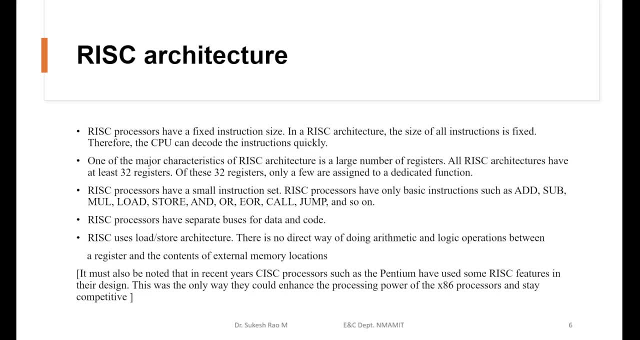 set which corresponds to 4 byte. So that is what the risk architecture Now, if you can see now why it is called risk. so that's one thing which, in the beginning of the class i told the avr is a risk microcontroller. so the risk is a reduced instruction set. 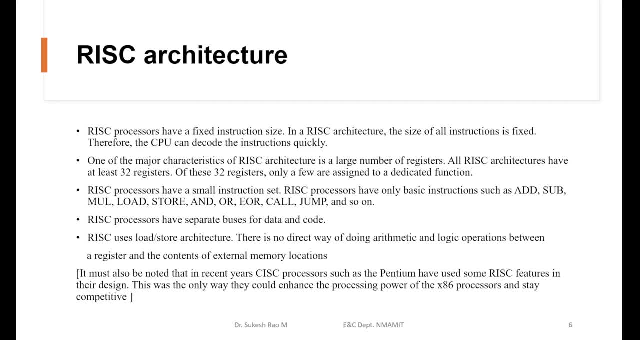 so here all the instructions will have the fixed instruction size either. it is always two byte instruction, in some case it is four byte, but they are multiples of two byte, so it is easy for the architecture to handle the execution time. we don't have a varying execution time, so precisely we can. 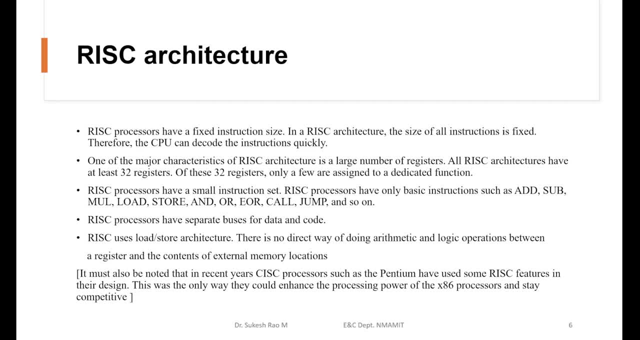 focus on the time. another uh factor here in the risk architecture is there is a large number of the registers. you have large number of the registers in the memory mapping there you can see that uh control registers. many things are there and apart from the 32 registers which are 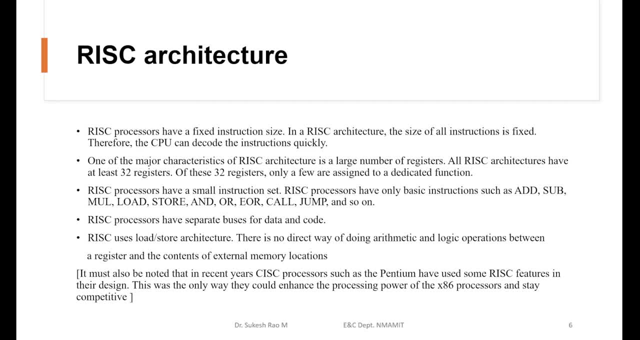 general purposes. okay, functional registers are there. they are used for, you know, configuring many of the modules. and in risk, uh, there are. processor will have some small instruction set. what i mean to say is there are limited instructions. you don't find much of the instructions here, so you don't have. 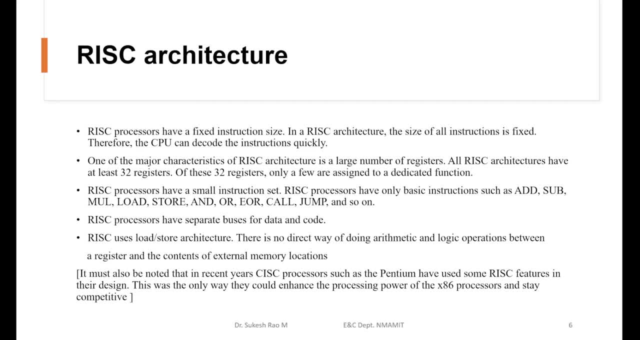 say: you know, uh, uh, risk processors will say: add some, you know, sometime the division will be done with the regular subtraction. you don't get a sub instruction at all, so they don't give any instruction which you can do it with the regular addition or subtraction. so some of the instructions. 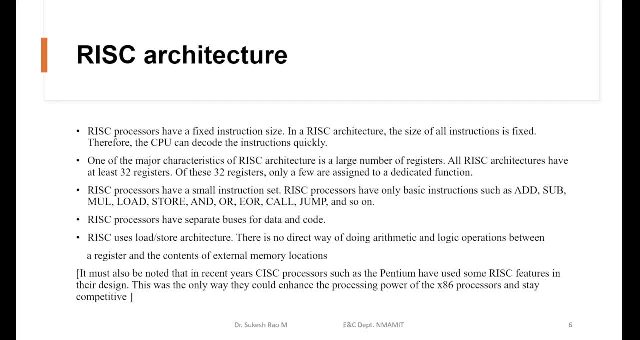 are not there. we have to achieve it with some random- i mean alternative- instructions and usually memory in the memory. data is separate, code is separate. you have a dedicated data memory. you have a dedicated code memory. that is a risk philosophy and that is also known as the passpoint or the data memory. that is a risk philosophy. 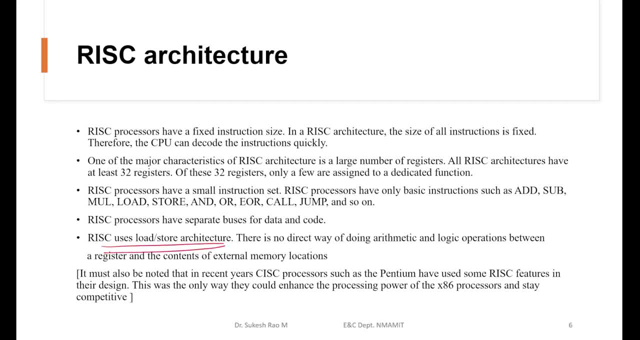 okay. so another thing is the load and store architecture. if you look at this load and store architecture- that is the point which is mentioned here- usually in risk anything that you perform with the memory in a data memory. if you wanted to add some number in the memory, 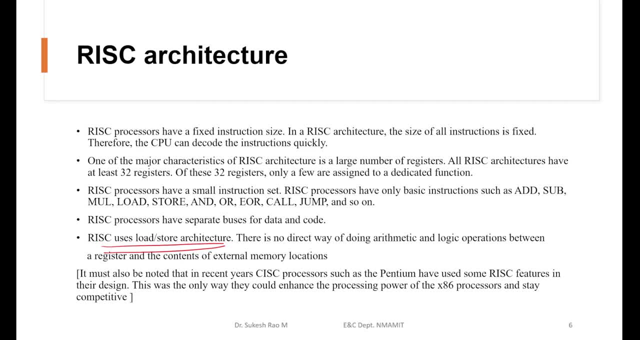 we can add it. So it is something load and store architecture. you do not. it cannot perform anything directly in that memory location, which is possible in case of some processor like 88SX, you know, Intel Pro Core, which is CISC based, which is not there in this. so it is a load and store. 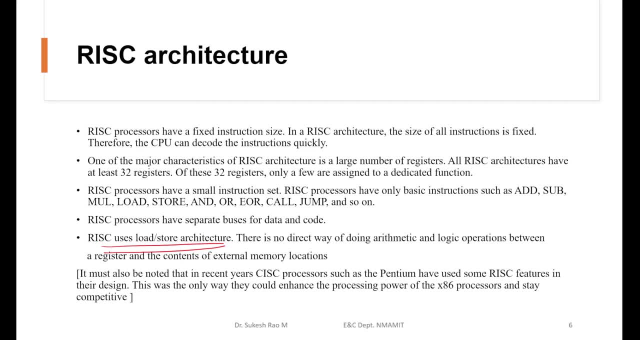 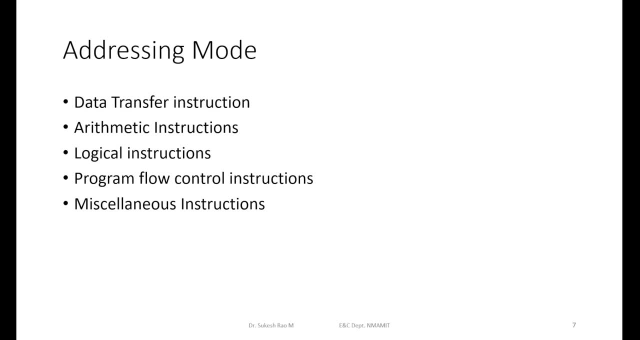 architecture, or usually some execution time is involved in it, that is, except that there is no other disadvantage. So if you look at this now, we will look into now addressing modes. So now, type of the instructions that we can. we can now learn about different instructions. 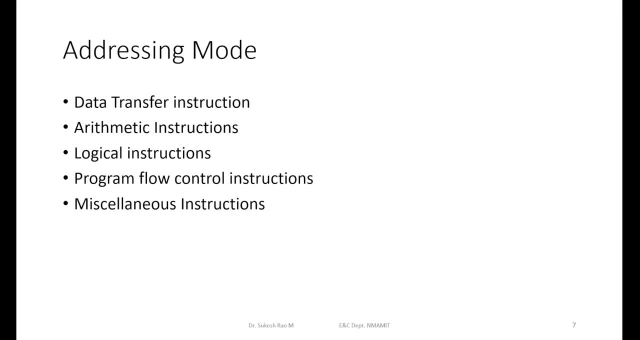 like, there are data transfer instructions, there are arithmetic instructions, logical instructions are there, program flow instructions are there. So data transfer instruction usually consists of some move instructions or load instructions. Arithmetic, you can find some addition, subtraction, you know, multiplication, all sorts of instructions. logical instructions usually consist of some rotate. 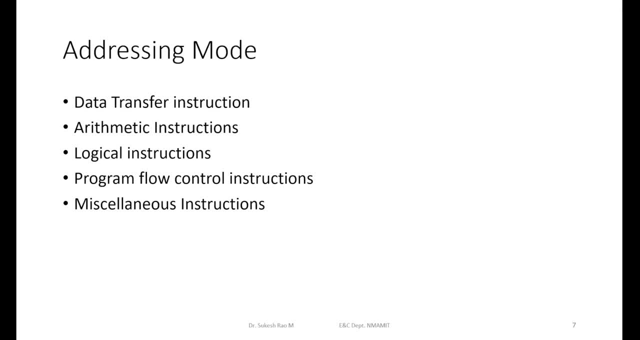 then shift and xor or and all set of bitwise uh logical operations, program flow instructions: uh, usually involves some looping. okay, if you wanted to achieve some looping algorithm, you can want to decrement and loop and check whether they are equal and loop. you know sort of instructions. are there miscellaneous instructions? uh, there are some. what kind of? 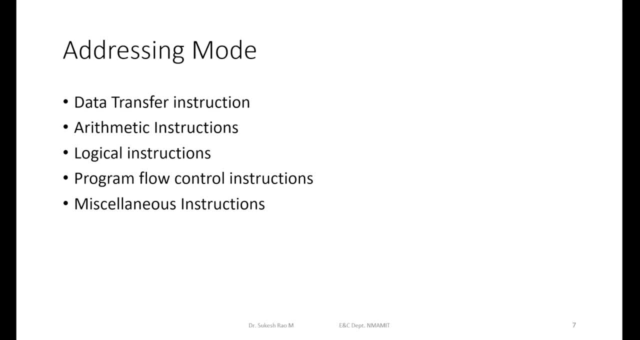 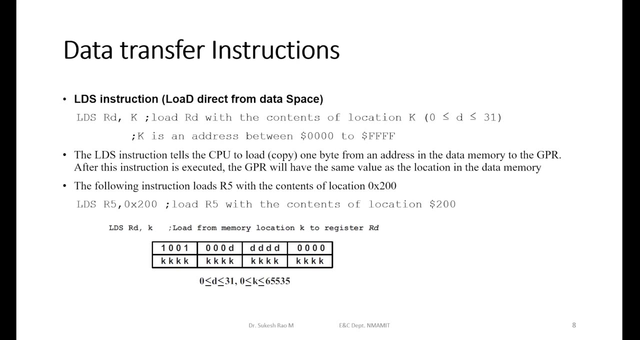 you know, swap or maybe setting some register high and low, clearing certain register. okay, this will come in the miscellaneous, so we'll focus on some of the instructions here one by one. so let's look at this: data transfer instructions. so we will focus on few data transfer instructions. 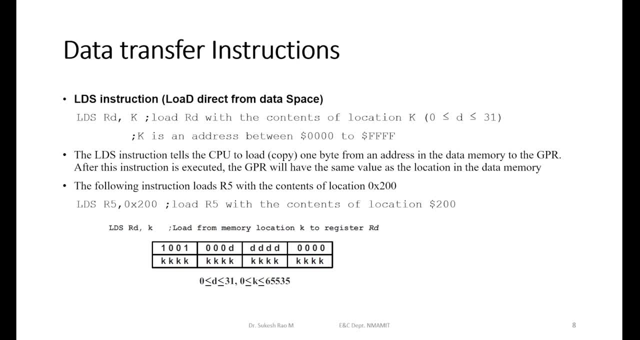 so that we can learn. you know how things are handled here. so if you look at the typical format- see format as instruction is given here- lds rd comma k. now i am going to use some uh, typical format with the textbooks also which i am referring, that is: 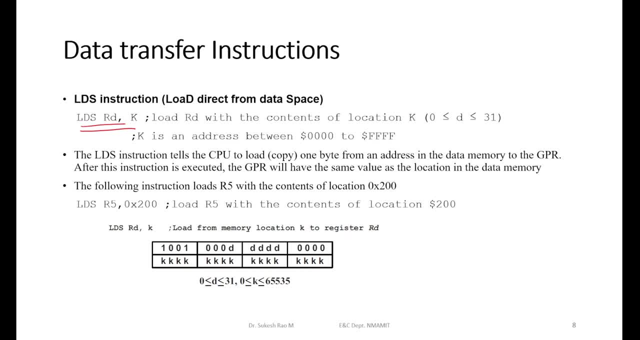 same way. so you can now make out which is operand, which is registers. so lds is a mnemonic for load direct from the data space. so you are loading something from the data space and rd is the data destination register where it is loaded and you can have some number. you see here You look at 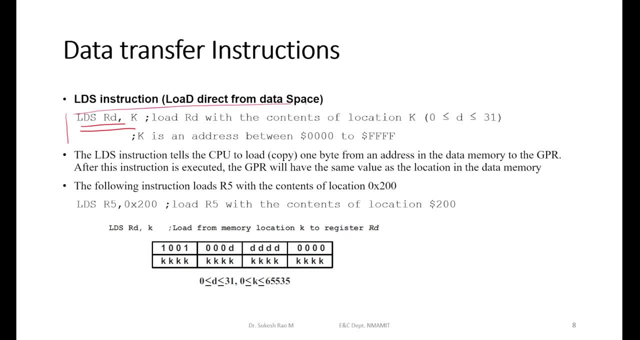 this is very precise information that you can get it from the data sheet. This is enough to understand what that instruction does. So if you look at this, load RD with the content of the location. what is that RD? RD is the general purpose register. How many are there? 32 are. 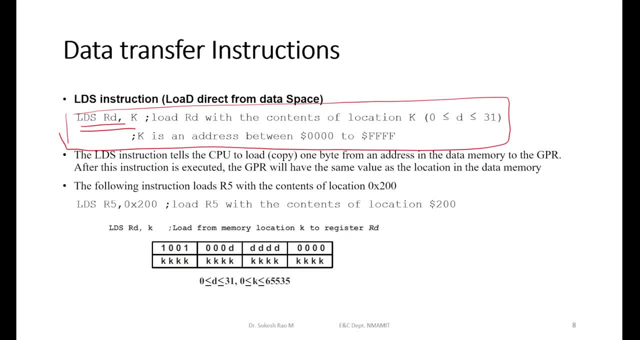 there, So I can use this with all 32 registers. What is the K? K is a 16-bit value ranging from this to this. It is quite easy, and what it does actually. Let us look at this. This instruction actually tells the CPU that you need to take one byte. It need to take one byte from the data. 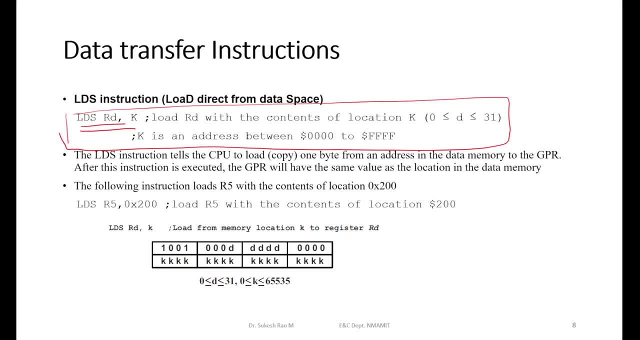 memory to the space. So what I am trying to tell here is, for example, this is the instruction Then from the data memory to the space. I am trying to tell here is, for example, this is the instruction Then from the data memory to the space. I am trying to tell here is, for example, this is the. 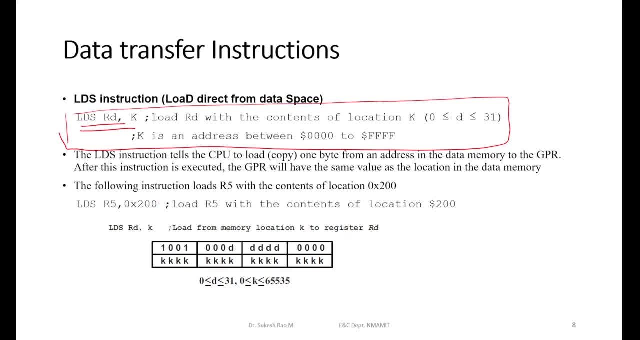 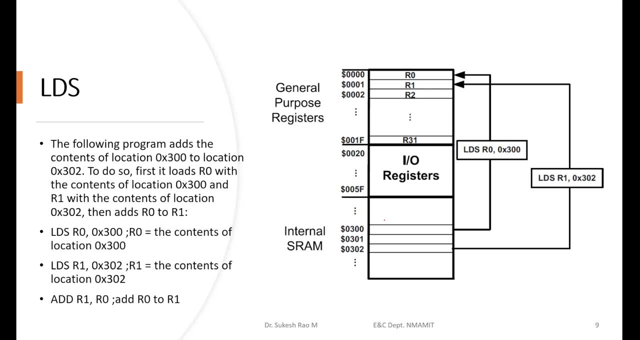 instruction. Then from the 200 location one byte value is saved. That value is actually loaded to R5.. So let us see, for example: 200 location is here. Somewhere you have say 200 location, here, 0 x 200. So it is having say content, say 77. Then 77 should come to R5. So R5 is here. 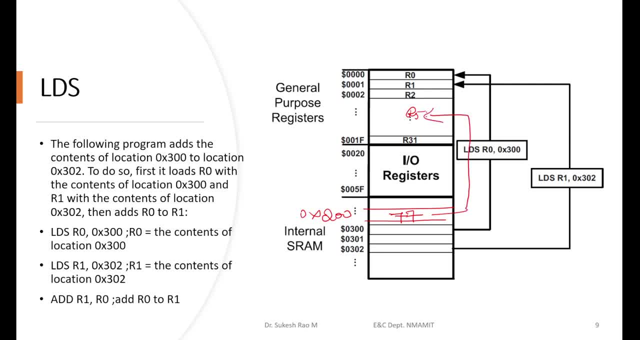 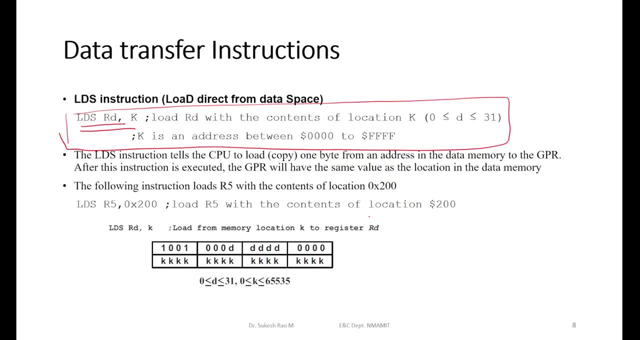 So what happens after the execution? LDS will save the 77 to R 5. that is what we are going to perform. Then look at this: LDS R D, comma 5.. So how it is coded. that is very interesting, I think, and as a computer engineer or 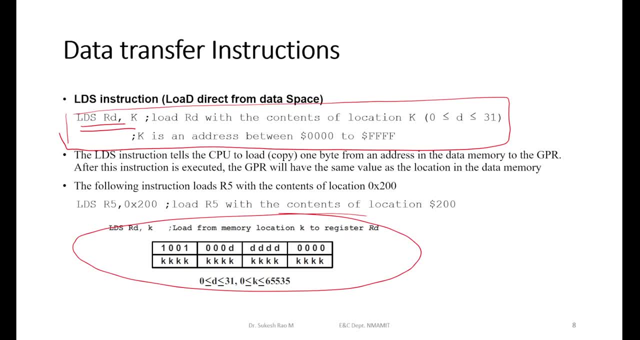 maybe an electronic engineer. we should know how the instructions are coded. that is very you know a fundamental aspect, rather than writing a program. So how these are coded, they use of optimum, you know usage of the bits available to code, because LDS has to be told you. 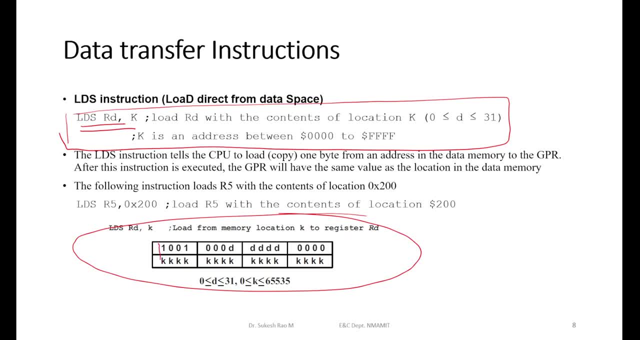 know what is that LDS? So this, if you see these bits will tell this instruction. it indicates, say, whenever it comes 1 0 0, 1 0 0 0, it is correspond to LDS. So LDS what and what? then rest of the parameter will be assigned. Now you can see here: R D is allotted with. 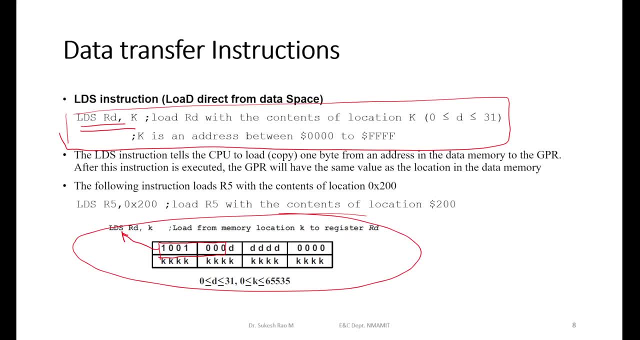 5 bits 1, 2, 3, 4, 5. Obviously with the 5 I can have 32 combination for 32 registers. So all that register could be mapped here and obviously this also will come. this also will come part of this LDS. only Now you have this, only then. rest of the number is actually next. 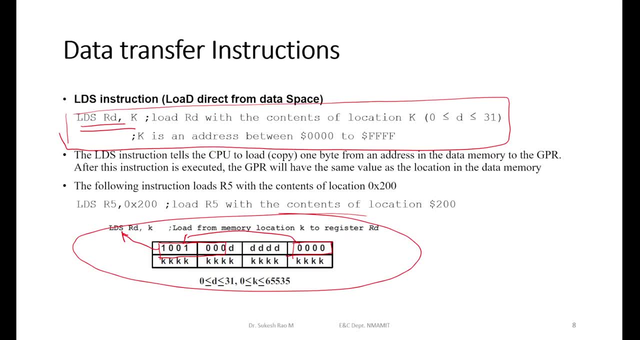 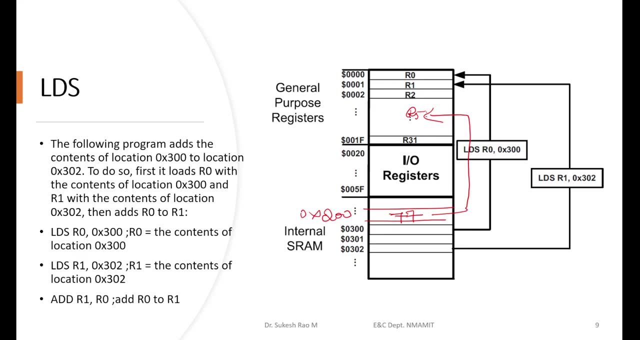 to K this. actually it is a. it is a. I think it is a 4 byte instruction. this is a 4 byte instruction because this value can range from 0, 0 to s, f. So if you, if you write here, if I am writing, let us say I think we 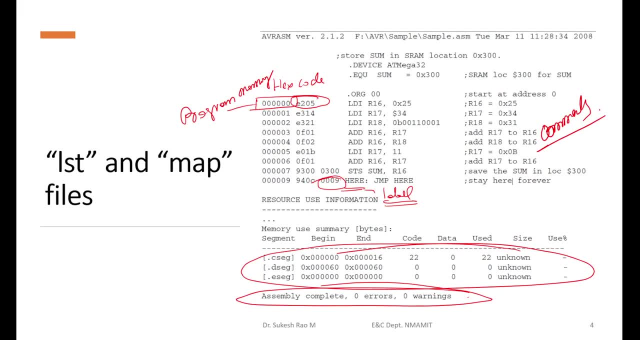 will go back to that example and just make out- I was just testing here, LDS. no, I have LDI here, So LDI, here I think, LDS. if I have to write, then I just write. So LDS, here, I think LDS. if I have to write, then I just write. So LDS, here, I think, LDS, here I think LDS. if I have to write, then I just write. 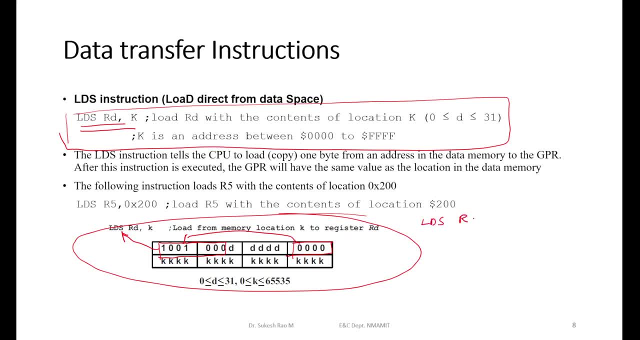 write, say LDS, R2, say 0x4000.. If I write then how it is coded, So it will be. so let me write here It will be: LDS is 1001000.. R2 is actually second register, So it will. 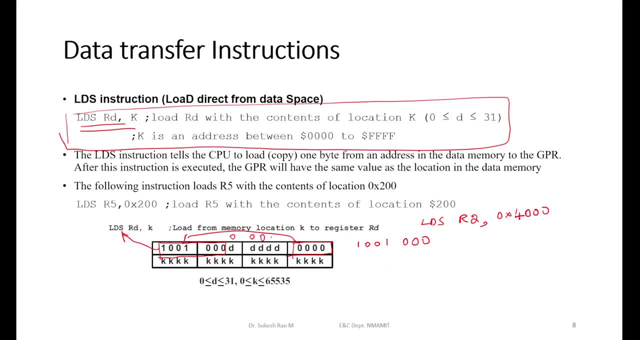 be 0010,, that is 2.. So this is 0010, then 000, as it is, Then 4 is there. So 0100, 0000,, 0000, 0000.. So this is 400.. So the instruction here it is: this is actually 9.. So this: 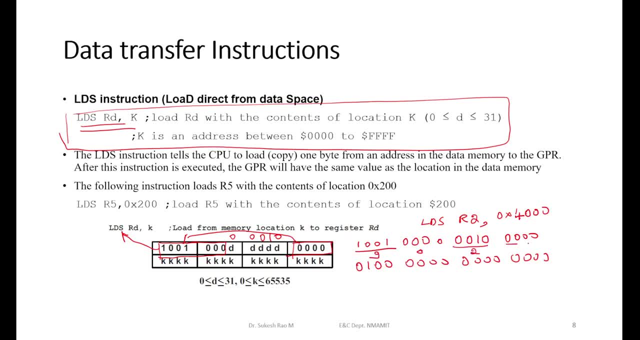 is 0000, 0000.. So what is that memory In the memory? 9020 in one location, 4000 in another location. So this is the opcode for LDS instruction. That is how we actually decode. 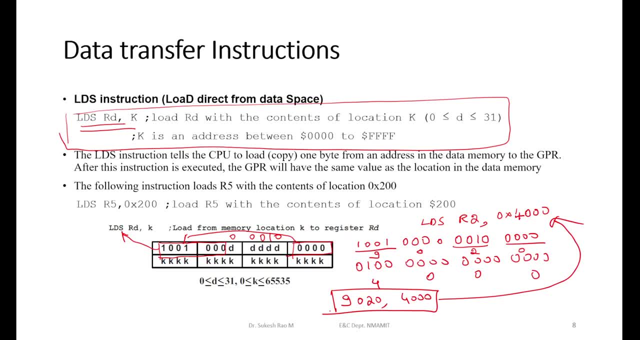 So you can just focus on this. I mean how? this? you can just get a general idea. When you look at the data sheet, you can get to know How exactly instructions are coded. So, as I- this is another example, you know. illustration. 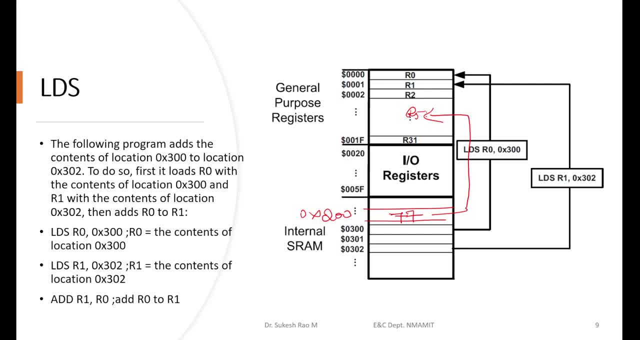 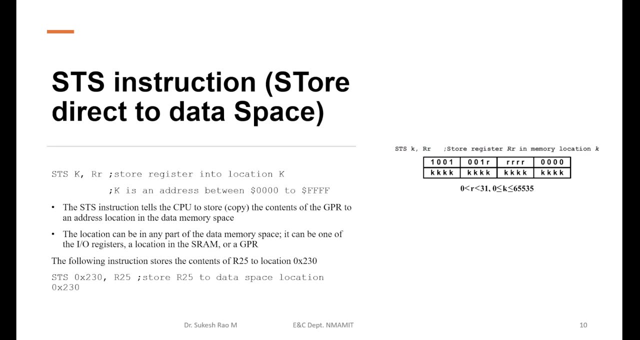 to give how LDS works, So for different registers, how the value from a memory is loaded. That's what this- So you can just have a look at this. Then there are other instructions- is SPS instructions. So SPS instructions also does the opposite way. It will store back. 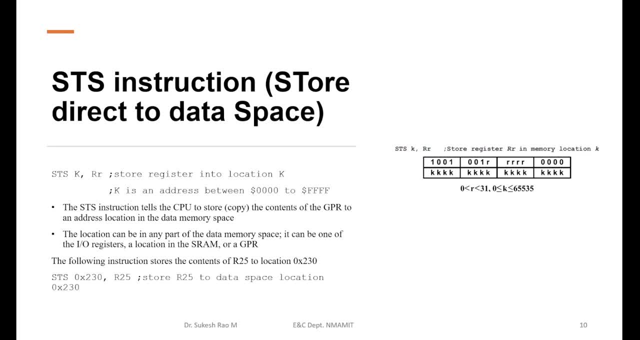 to the memory location from a register. ok, So if you want to store back to a memory location from a register, uses STS instructions and the format is given here. how it is, the locations are actually, you know, saved here and you can get the values. 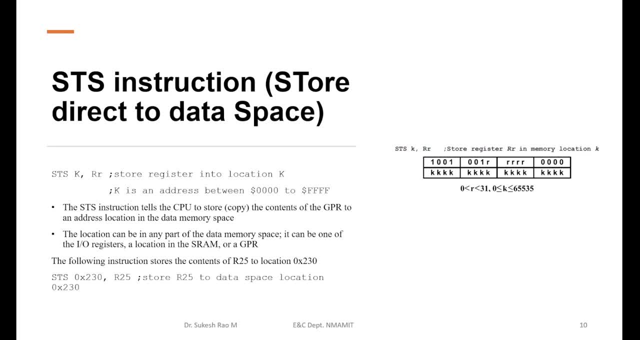 So let us take up this example once. I will give again how this STS is. you know, look at this STS 0x230, comma R25, correct? So this is the one. Now what it does. actually, the content of R25 is loaded to 230.. So how the instruction is loaded into the R25.. So the 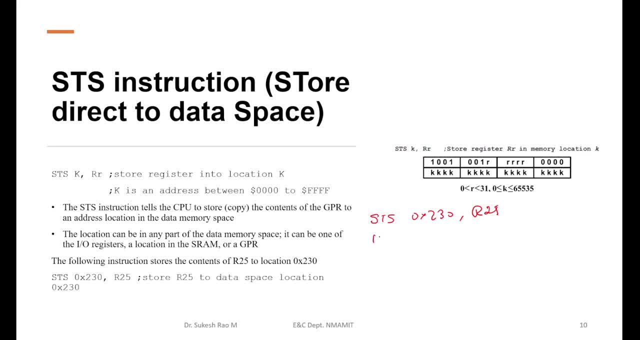 are coded. Let us have a look at this. This STS is 1 0 0, 1 0 0, 1.. Then you have actually only 4 bit. you see here, only 4 bits are there. So I think 4 bit means the yeah, it start. 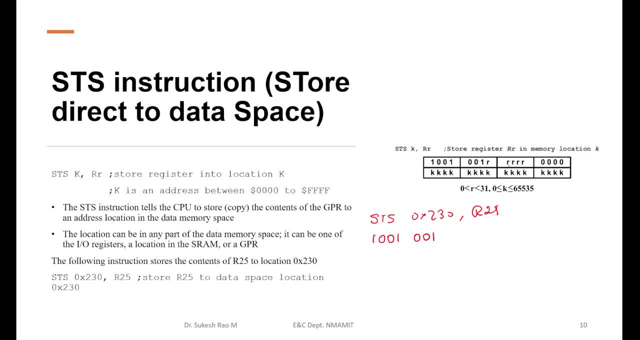 from 16 actually. So here only, sorry, 4 plus 1, 5 bits, are there? anything can be fine. So what is 25? 25, the binary you need to write. So it is actually say 8 plus, So it is 16 is. 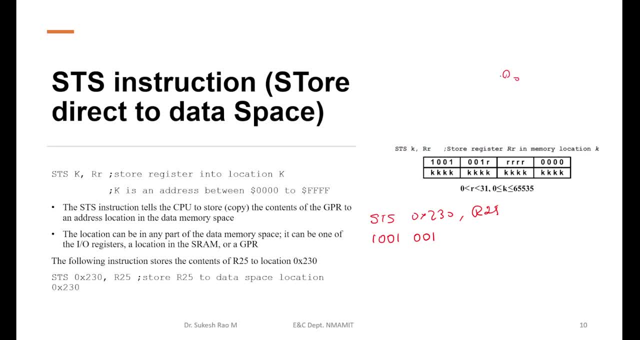 so let me have d naught: d 1, d 2, d 3, d 4.. So this is 16, 16 plus. I should actually perform this conversion from this 25 to you know the binary conversion- so that i can fill that value. 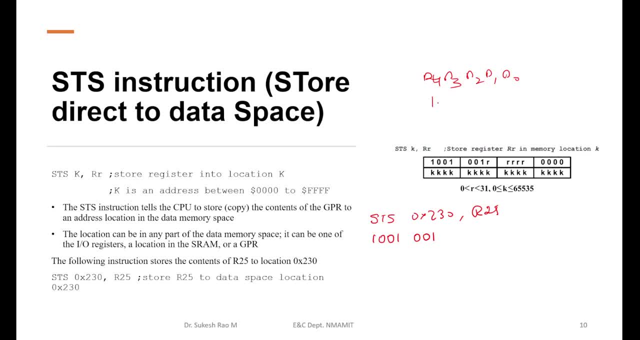 so it will be 24. so 16 plus 8 plus 0 0, 1, is this okay? so this is actually 8, this is 16. this is 1, correct, 24.. so this is 1 0, 1, 1, 0, 0, 1 correct. so the values here. 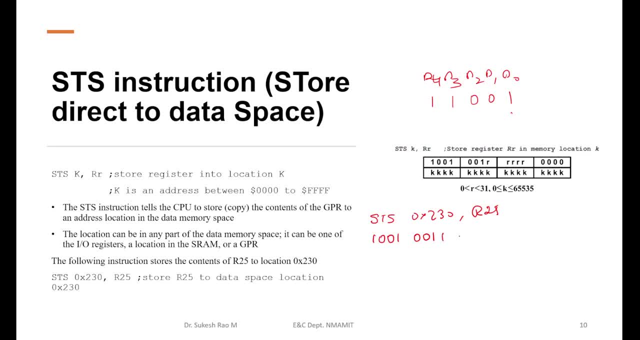 so 1 0 0, 1 0 0, 1, then 1, then 1 0 0, 1, then 0 0 0, 0. k is what? k is this much: 2 3 0. so 0 x 2 3 0. 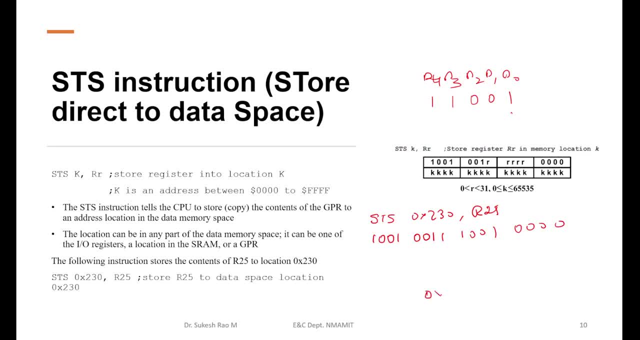 so obviously, this should be written as 0 x 0, 2, 3, 0. okay, because it is a four digit, so you cannot append a zero in the last. it's supposed to be on the left side, so 0 0 0 0 and 0 0 1, 0 0 0, 1 1 is 0 0 0 0. okay. so obviously, and as it is, i'm writing the hex. 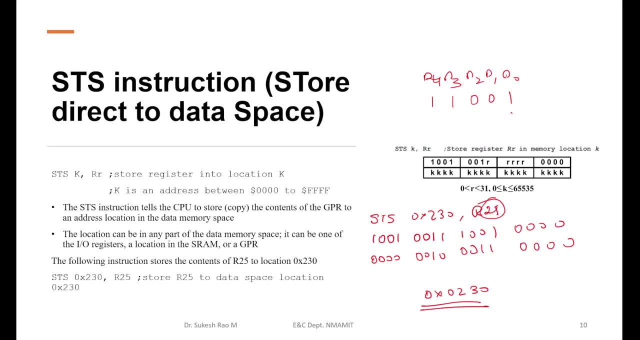 number because it's already given in hex, whereas this is in the decimal. okay, so i should convert it. so this is the opcode. you can just look back to the bits. you can just write this instruction and compile it. i can just show you some of the- uh, maybe in the lab tutorial. i can just show you. 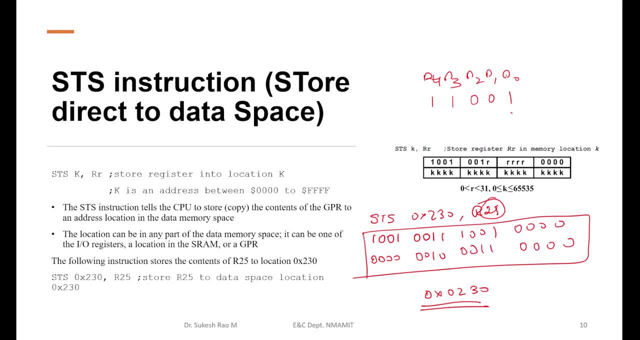 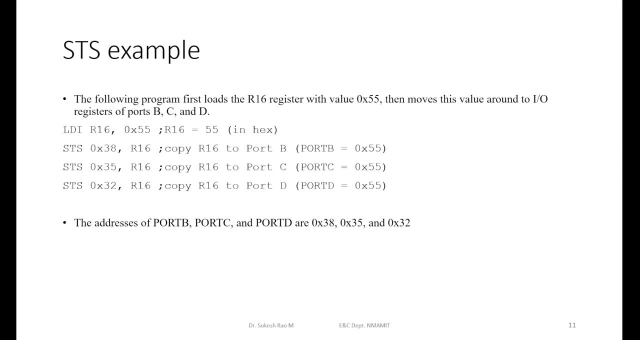 how to see this. okay, maybe in the couple of days i'll just give you another, so sts example is given here so you can just have a look at this of how what it does. so, uh, what is the program? first loads this value where i say r 16 with 055 value, then moves it to the value around to the io. 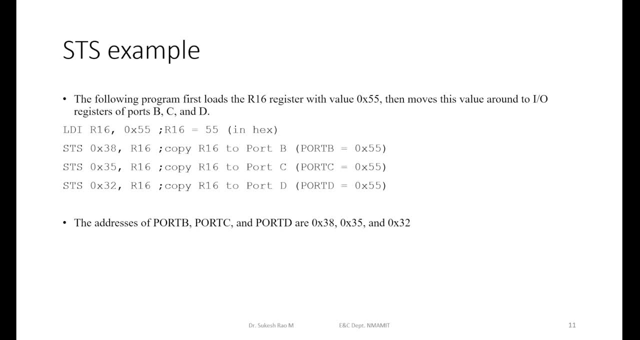 register of 4, d, c and d. okay, now, if you look at this, first to load the value 55 with 50. so this is the instruction i used. that's perfect. then i will be loading, then move this value around to the i. so r 16 is. 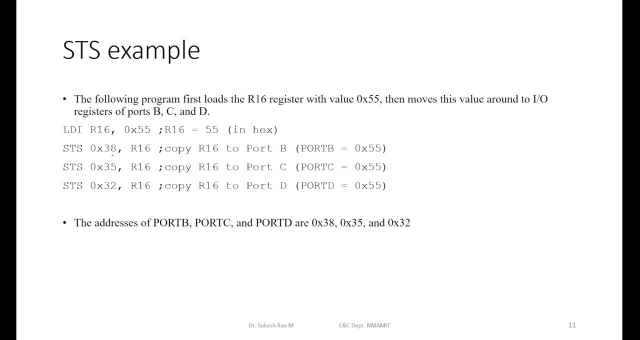 that I supposed to load it to some of the register here, which is actually the IO register. ok, So how do you know which are the IO registers, the address- I should know the address here. So how do you know that address? So you should have refer to some memory map here. 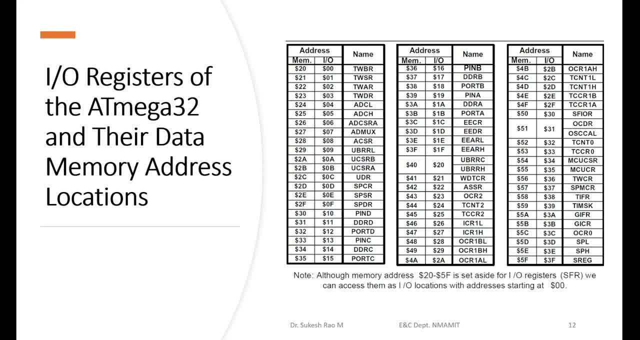 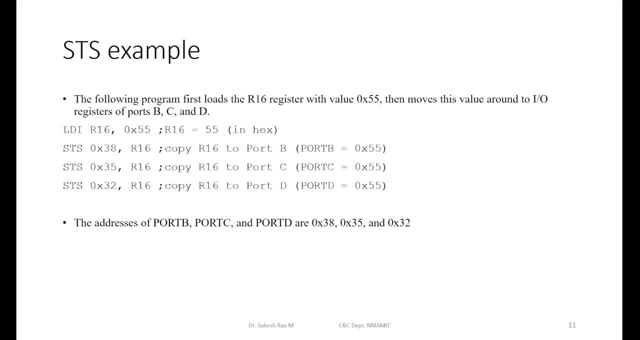 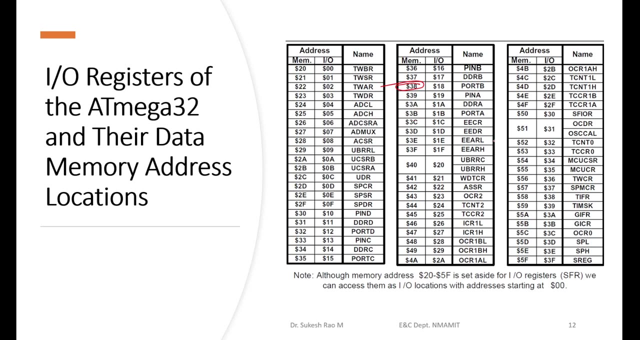 So look at this, So here you get. you see, here, this is 38, port B and port A is somewhere here. ok, where is it port A? yeah, yeah, it is here, port A, port B, and what else is asking port? so port A is not there. port B, C, D, ok, So anyway, this is not there. port B, port C, I found. 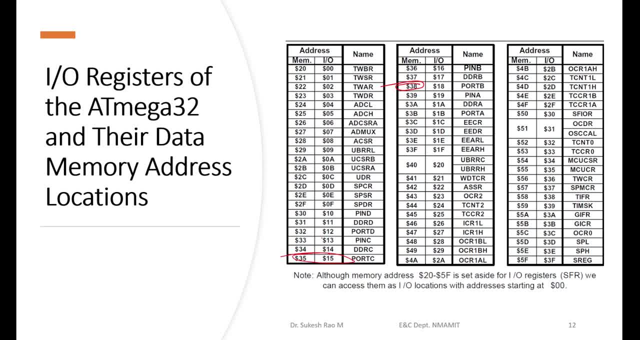 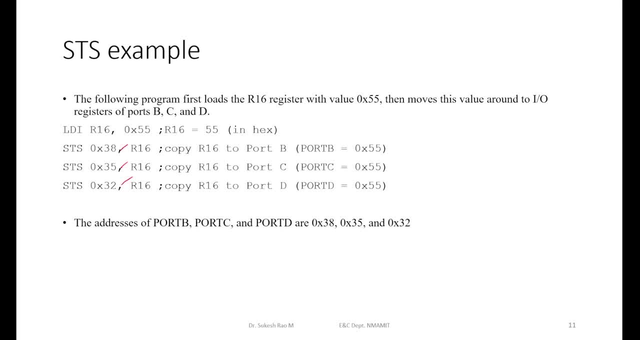 it somewhere here and port D is here. So you look at 32, 35 and 38, 32, 35, 38. see, this is the location. So if you write this location, that is enough. Otherwise, if you have another instruction where you can straight away write port B, port. 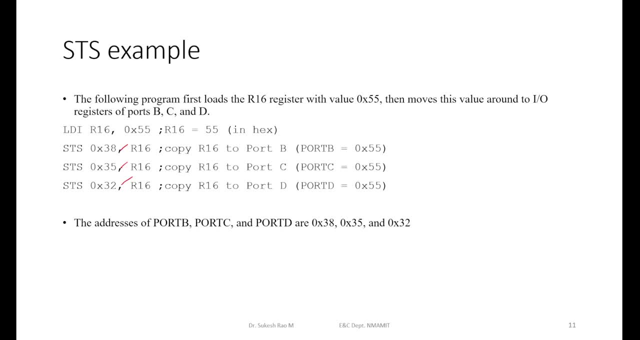 C port. ok, you can do that. So this is another way of moving the value to the port from the memory, like I moved it to a register. from the register those values are load to the port. that is how this can be illustrated. So this, if you see carefully, observe here. 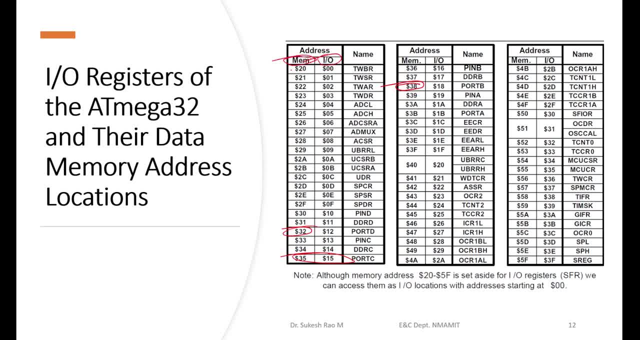 in the memory. you have this memory address and IO address. they are two different things. one starts with 20, another starts with 0.. Now there is a reason. if you look at the memory map you come to know why it is 20, because previous to this, I think, some registers of R naught to R 32 are there. that is why this. 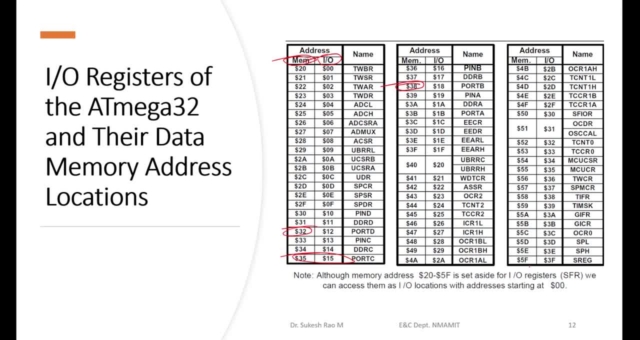 is start from 20, from 20 to it goes till, I think, here, 5 f. ok, all the registers are there, apart from that IO register. you can see something over here. ok, Now these registers are can be accessed. in the special instruction they specify IO location. 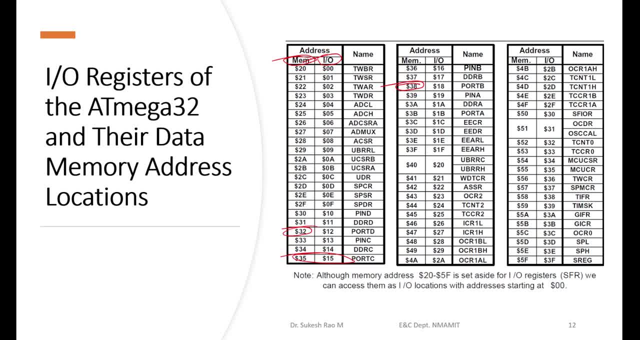 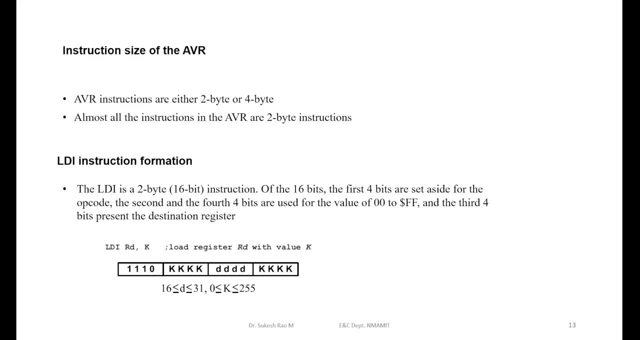 you should use this So generally. location: if they give, then 32 is for port B. if they say IO address, then you should write A, 12.. So we will have a look at that instruction when it comes The instruction size of the AVR, I already 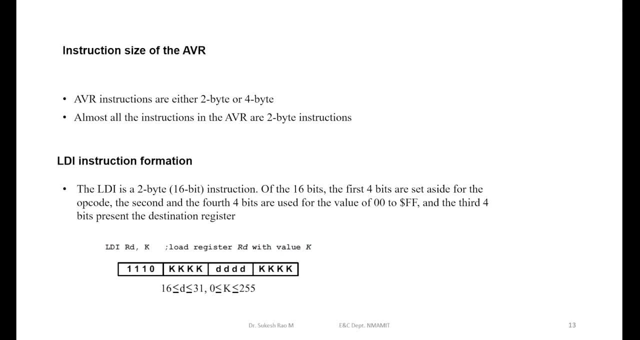 mentioned you, there is no 1 byte instruction. it is always a 2 byte because it is 16 bit. one single instruction or it can be 4 byte instruction. most of the instructions are 2 byte. So LDI instructions, loading some immediate value, any immediate literal value, if you want. 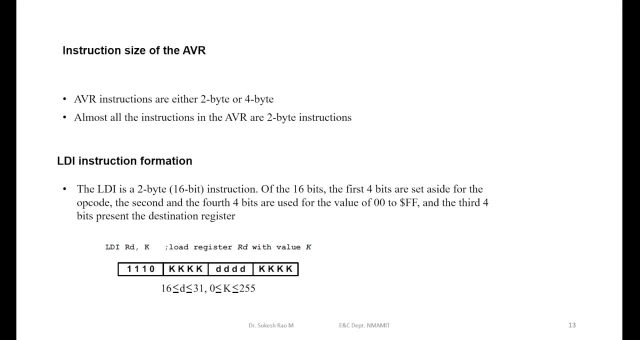 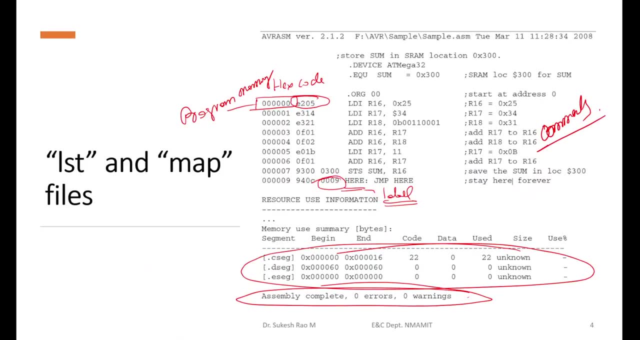 to load. you can use this LDI instructions. So I think in a couple of time back, I think we have seen this LDI instruction. just recall this instruction. see, here is an LDI R, LDI R 16 25. you remember this E 205. I will tell you how that E 205 came. So it is actually. 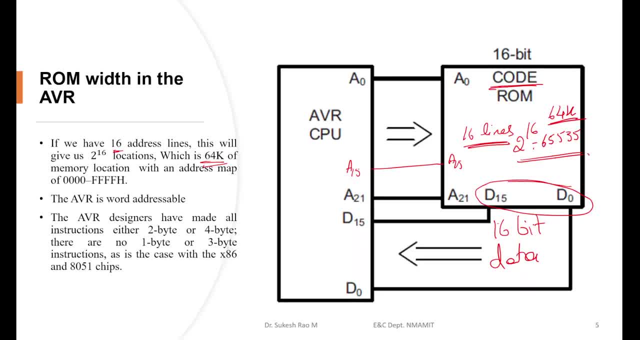 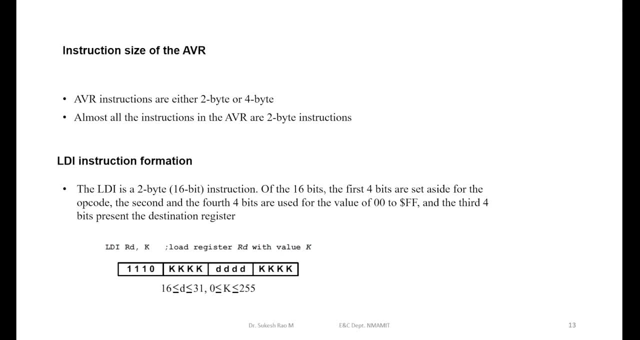 machine language. So how it is within LDI R 16: 25.. So let us go back here. let us look at this instruction. what this says is: this LDI instruction is loading us 16 bit. sorry, yeah, it is loading a 8 bit value that are loaded to the register. those values can be from 0, 0 to FF. 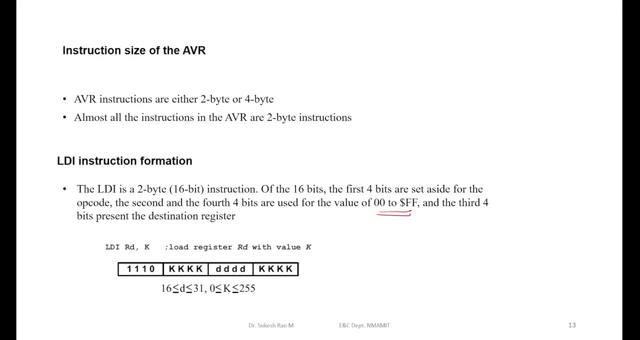 And in this it is a 16 bit instruction and they are actuallymaking it the rest of the bit they are configuring for loading the register. I mean addressing this. all these mapping, these values, they do. Let us see how they did it. look at this instruction format here: 1110. 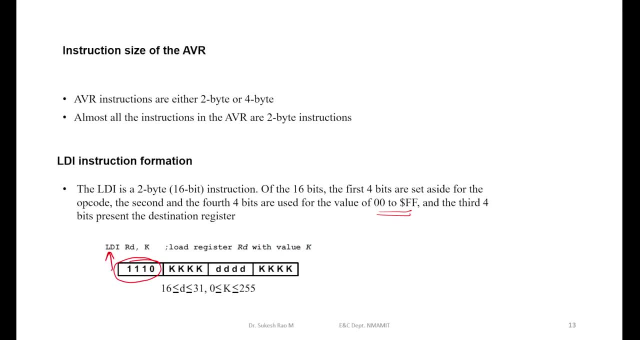 actually, this is dedicated for to understand. this is LDI. If they find 1 1, 1 0, then it is automatically loaded to the register. So let us see how they did it. So this one is one one, one, one zero. actually, this is dedicated for to understand. this is LDI. if they find: 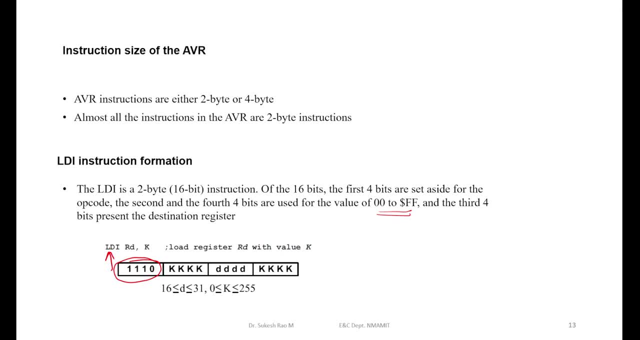 one, one, one zero, then it is automatically loaded. So let us see how they do it. So let us see to decode it as LDI. What is RD? Look at this value. This bit is RD. There are only 4 bit. 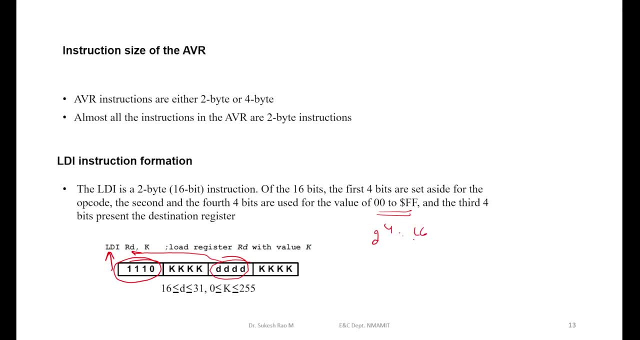 then that means 2 to the power of 4 is 16.. So you can address only 16 registers. So what are those 16?? That starts from R16 to R31, only this much You can address. 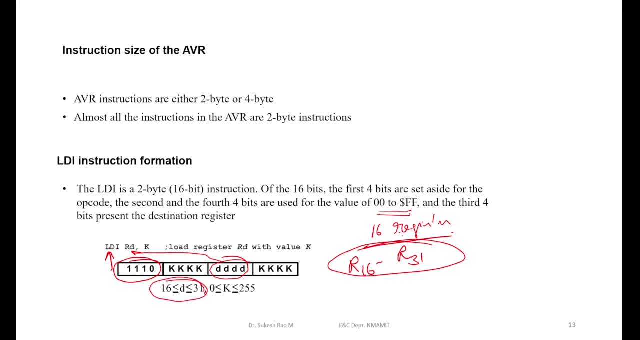 it is given here. you see here R16 to R31.. Then these are the 8 bit value that is referred to this. Now let me write that LDI R16 comma 0x25. it is right, Now they have written. 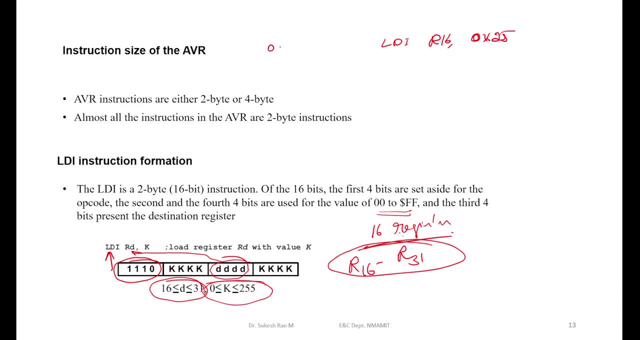 it in this way. Now, what is that? E? I think it was some value which came, I do not recall. Let me derive it here. So it is 1, 1, 1, 0.. R16 is. 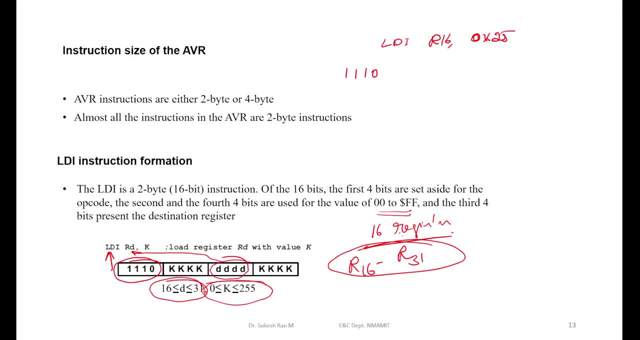 actually starting register, So that is 0, 0, 0.. R16 is the starting register for this set, So it is 0, 0.. D is actually sorry, K K This field, then third field, I will fill 0, 0, 0. 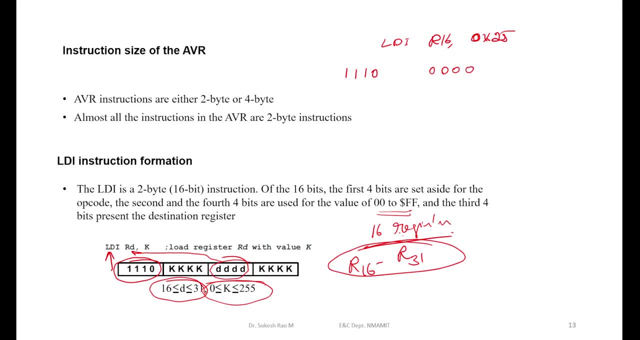 That is R16.. Then K is what 25, no, 25 is hex value, So it is 0, 0, 1, 0 and 5 is supposed to come here: 0, 1, 0, 1, correct. 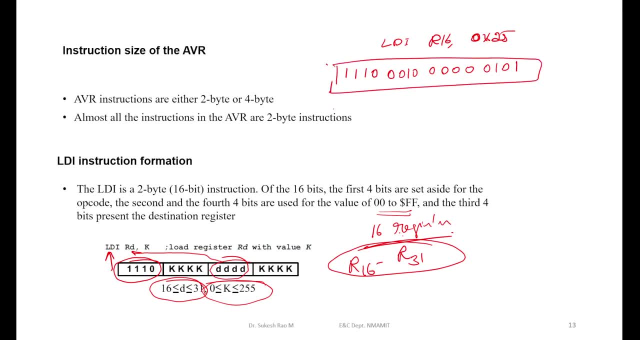 So this is the entire instruction code. What is it? E 2, 0, 5.. This is what you have seen there. E 2, 0, 5 comes with this way, As it is a single 2 byte instruction. this is the code for this. 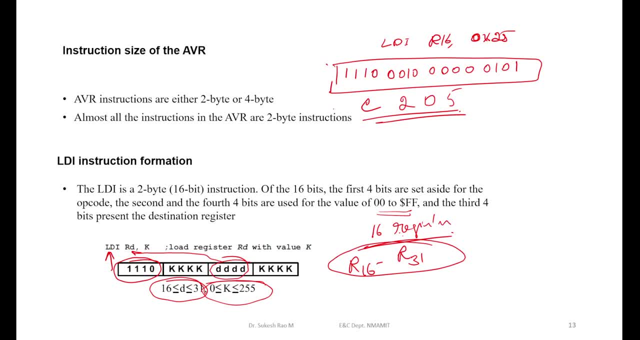 So usually you need not have to do this. It is. it is performed in the assembler itself, But you should. you should remember you know what is the logic used and how the instructions are coded. That is very important thing to learn here. So this is about the LDI and operation. wise, I do not find it any 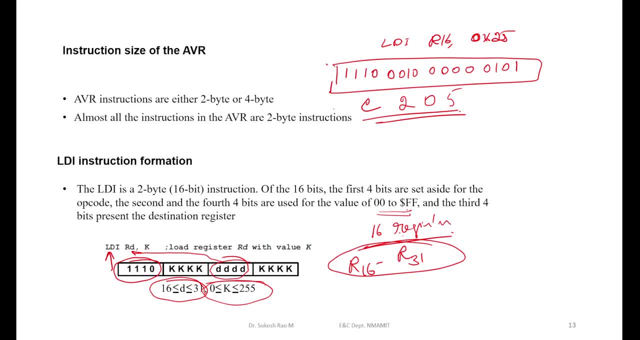 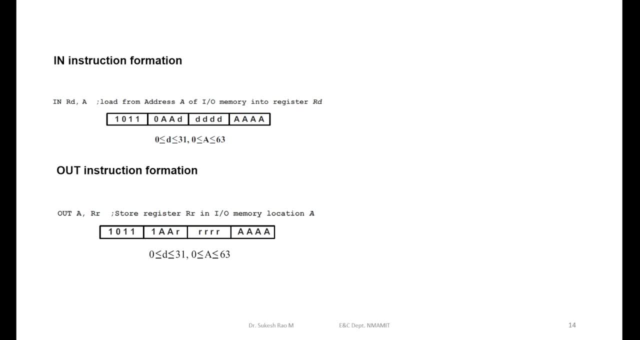 difficulty here because the literal value 0, 0 to FF is loaded to that register, R16 to R31.. There is a in and out instructions you can see. In is specifically you see here: look at this: This one line is enough to understand what that instruction is. 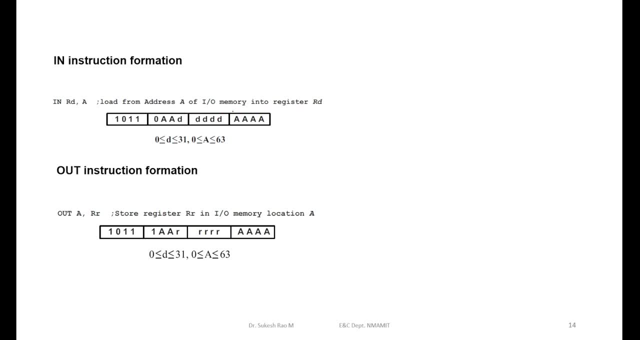 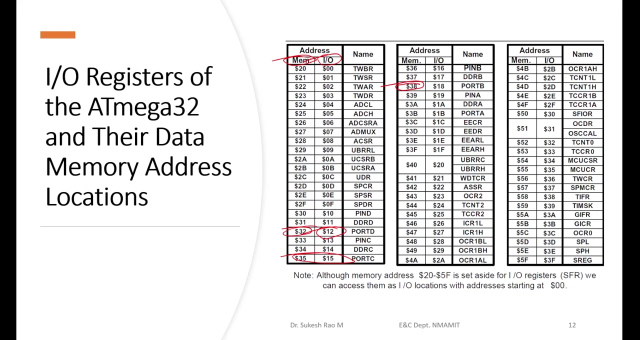 Load from the address A of I-O memory. Remember I-O memory. So you are loading something from the I-O memory into the register Rd. Rd is given which says all 32 are accessible. What is that? I-O memory? I-O memory is different. What is that? I-O? Look back this. 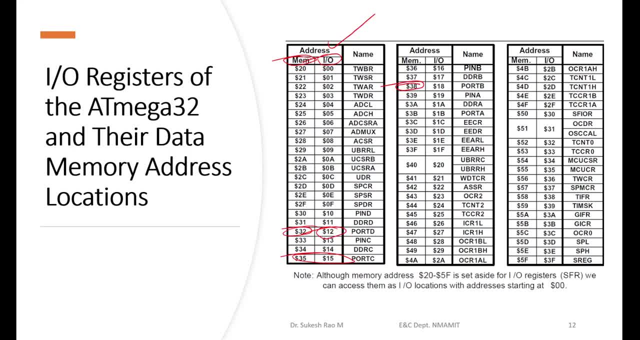 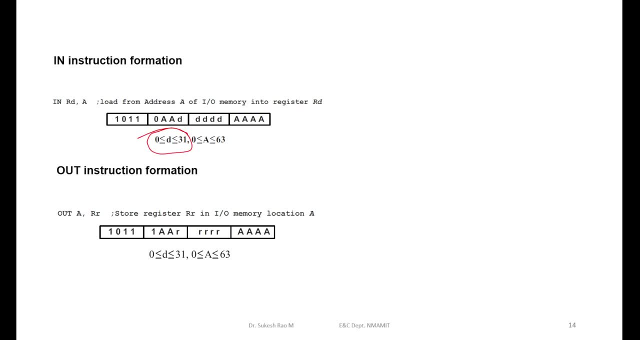 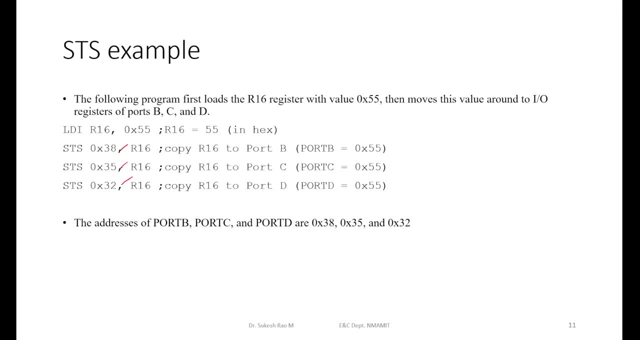 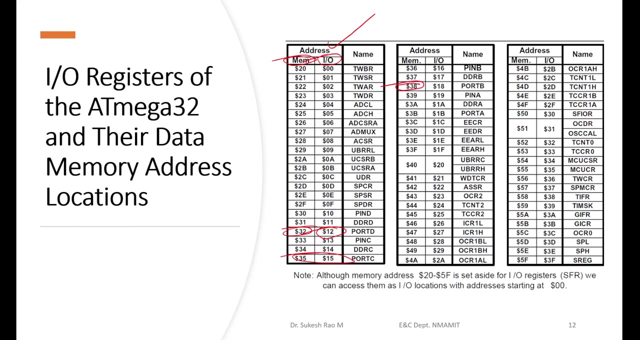 to write something for port A, then you should be a different address. It cannot be the address which I gave in the previous thing. So for this you wrote 32,, 38 for port B here, But here port B- if you look into carefully- 38 and 18.. So here when it comes, it is in. 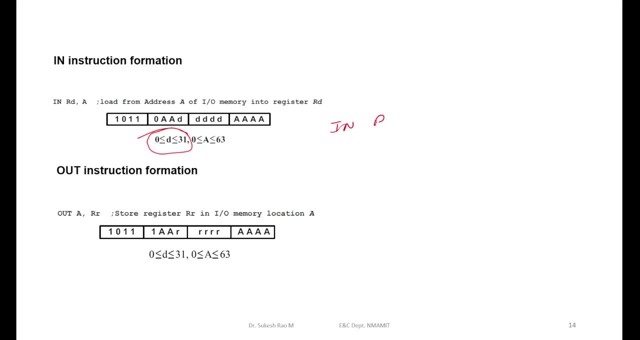 then Rd, Rd 38. So in Rd, Rd means here it could be any register, So say R20. And if you are reading it from port B, then I will just write it as 18.. 0x18.. That indicates that it is port B. So you just have to write either port B, because 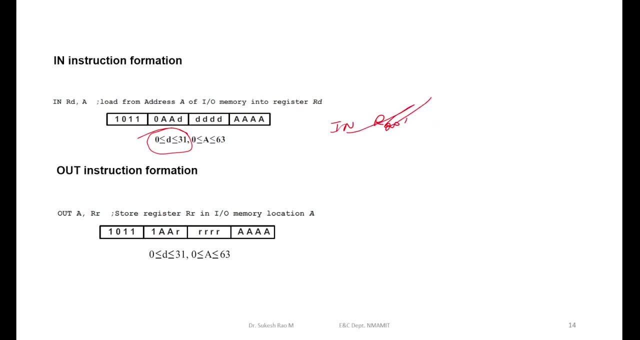 sometime assemble will take a conversion here, So but this is the format. In instruction always loads the value to the register from the port. that is in And out instruction is port from the register. So that is what in and out instruction. So you may have to.